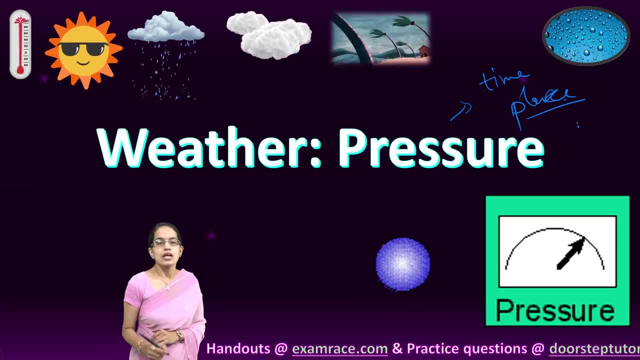 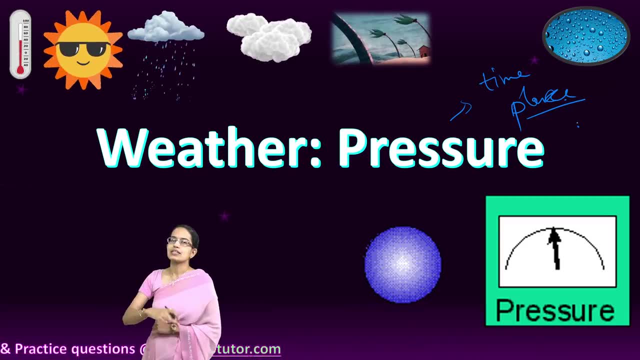 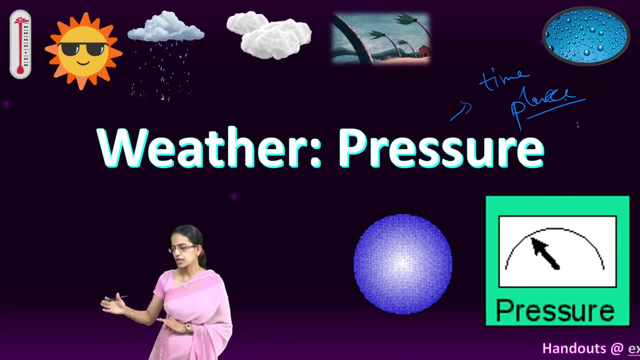 the, the, the pressure would vary. now this also occurs due to differential heating. differential heating means the land and the sea. let's take that example now. wind movement would be caused because of the differential heating and this transport of the heat and moisture would take place and ultimately, 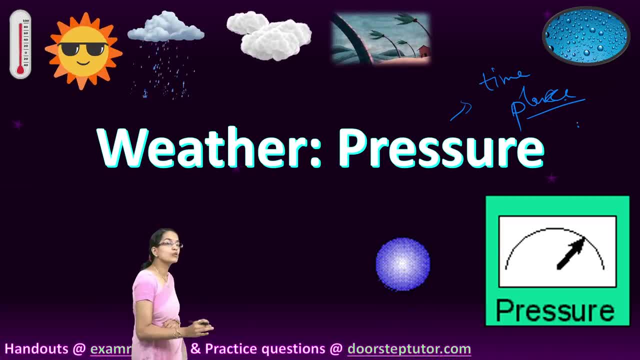 the pressure would be determined. pressure is also determined by density and temperature. now, pressure is also determined by density and temperature. now, if i am close to the ocean or i am away from the ocean, whatever temperature's been measured, plus what's happening at any of the sun's surface, 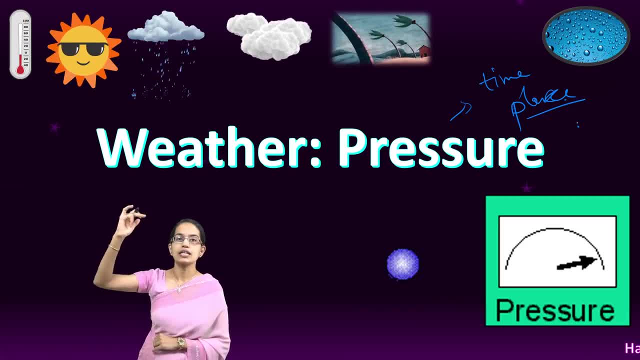 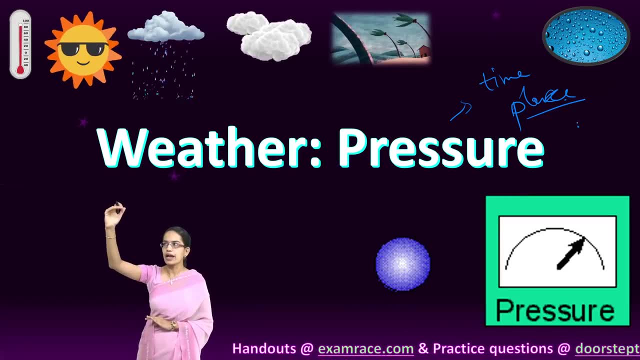 whether the temperature is hardly changing because of the temperaturehando. if it's high, you'll find that in the geography the atmospheric pressure decreases down. ie the friend of that question says the temperature is convinced. Dear students and friends, we know, and previous studies have shown, that number of 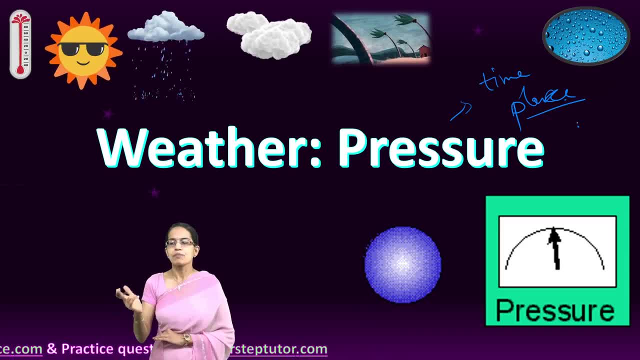 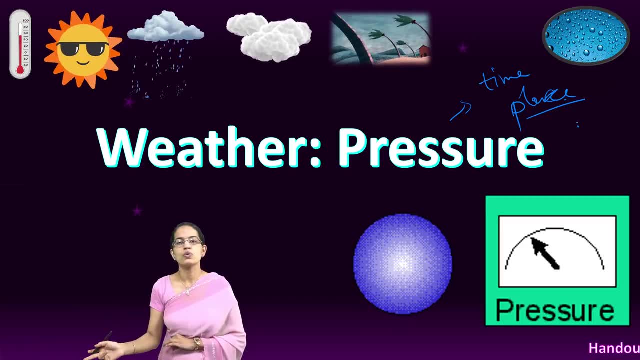 it in favor. the temperature decreases and of course the atmospheric strength decreases. it decreases frequently above an Pedal isасть, some people say because there's a phwas. at the time of when i ammodified, the pressure wills, because it usually changes from speed to force. ie five to six k meng is equal to the number ofrelations, so Ul thekus of pressure. 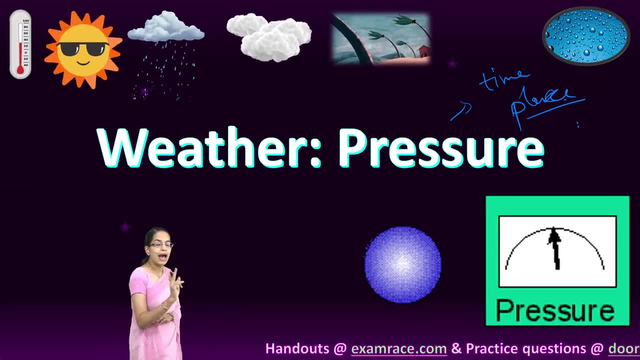 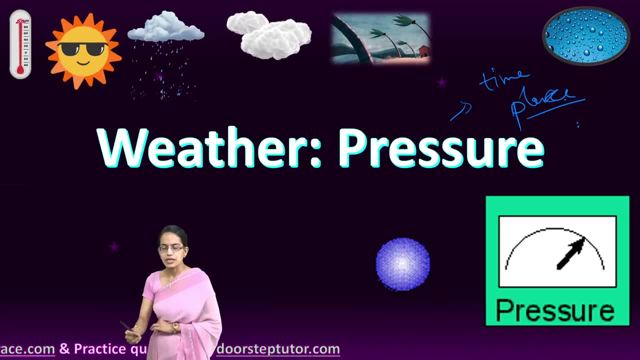 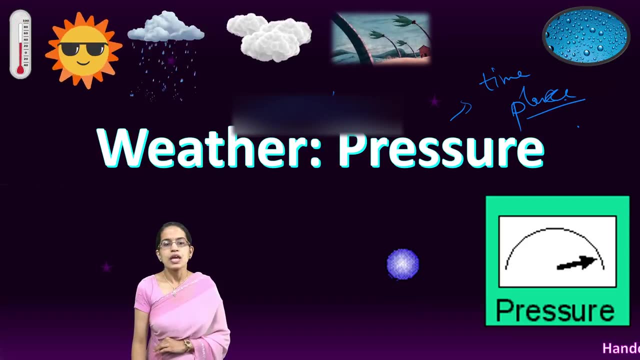 pressure increases if the temp is appreciate, so it's simply decreases as you increase in height. this pressure is measured through barometer. temperature, as we understood previously, is measured through thermometer. pressure is measured through barometer. So standard weather pressure, we say, is 1034 gram per square centimeter, and this is usually 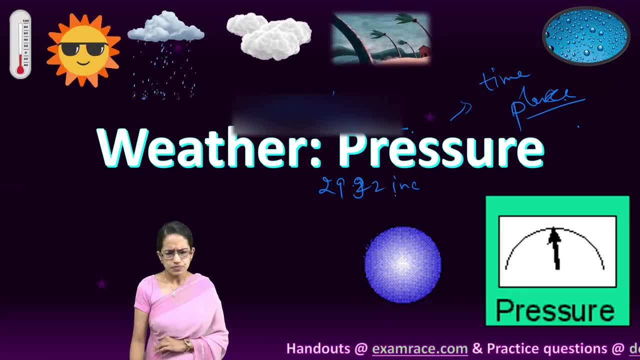 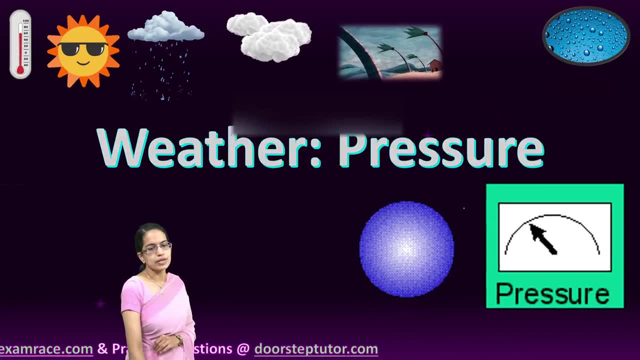 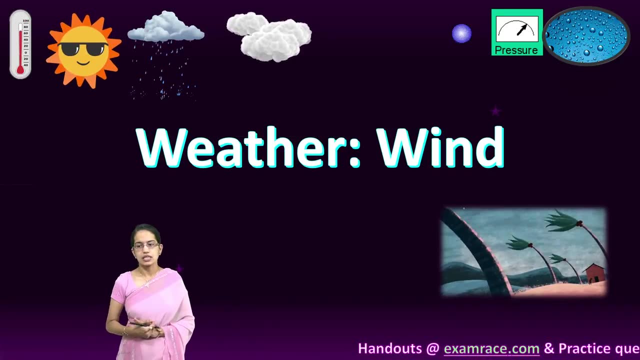 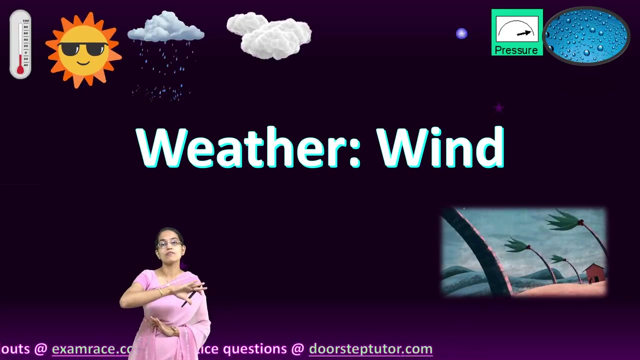 given at 29.92 inches, or we say 76 mm of mercury column. So those are the basic criteria based on which we have the pressure. The next is wind. now the direction of the wind affects the temperature. winds usually move from warmer areas. if they are moving from warmer areas they would increase the 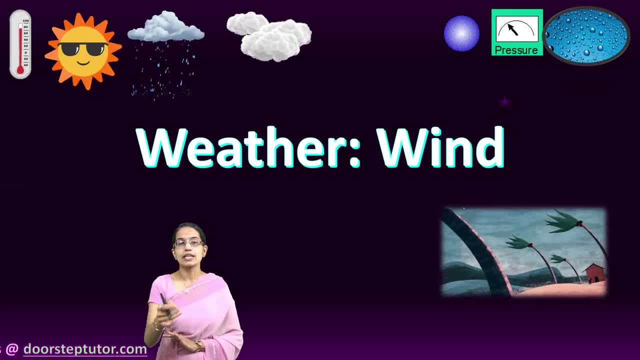 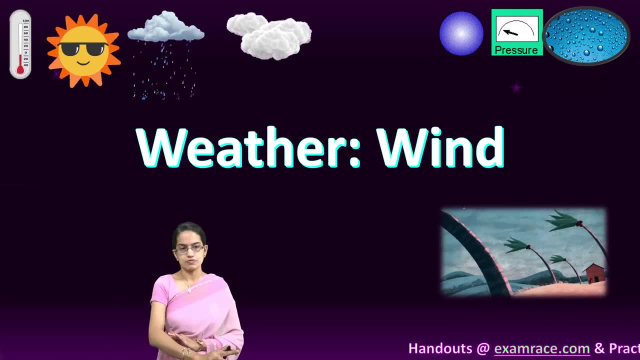 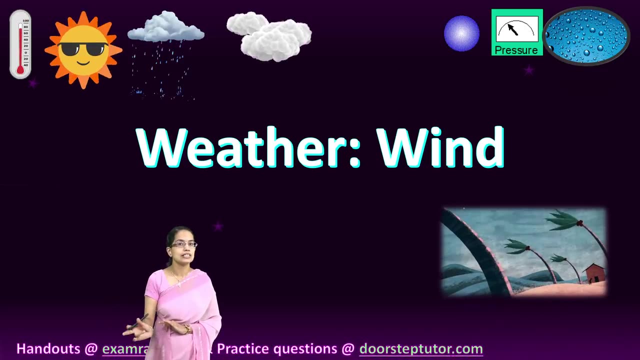 temperature. if the winds are coming from cold areas, they would decrease the temperature. So wind has a significant impact on the temperature of the region and is an important factor in this. Now, wind direction and speed of wind, both of those are analyzed through the weather. 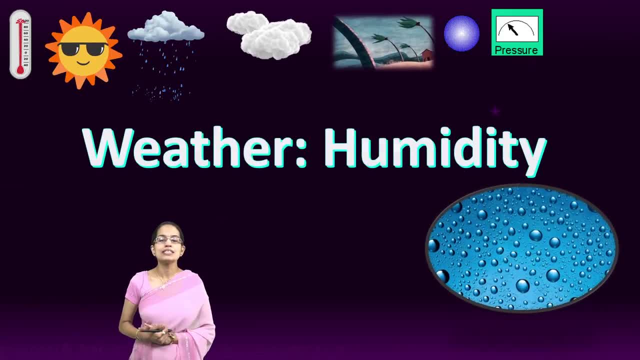 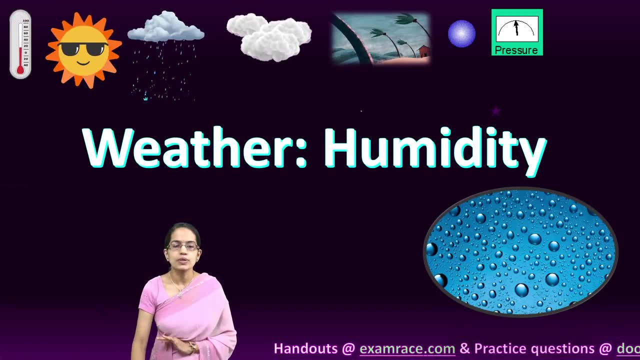 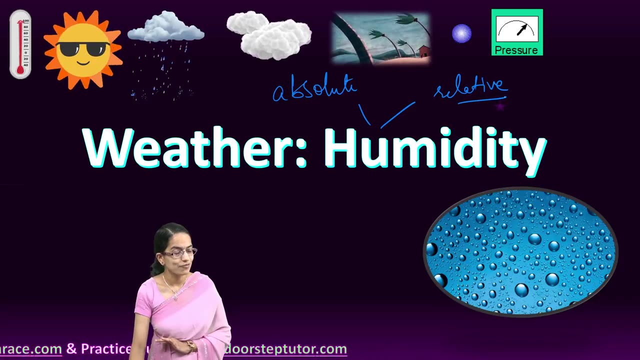 instruments which we would understand in the next section. The next is humidity. now, humidity is the amount of water vapor in the atmosphere. So this humidity can be explained as either absolute humidity or relative humidity. what is the difference? Relative, since it is relative, A related to B or A in contrast to B. 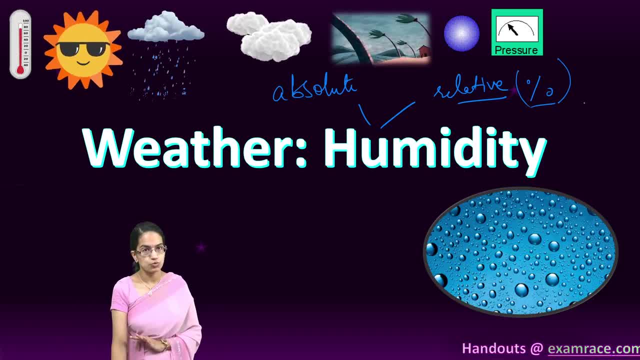 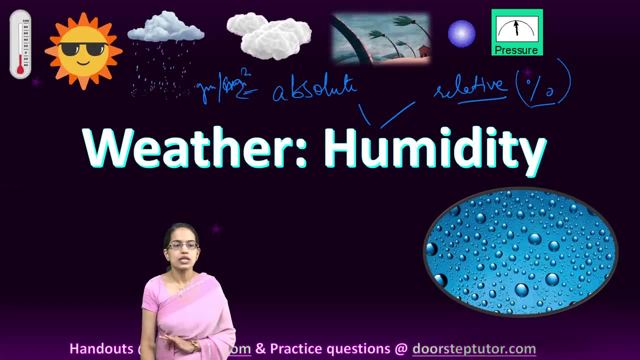 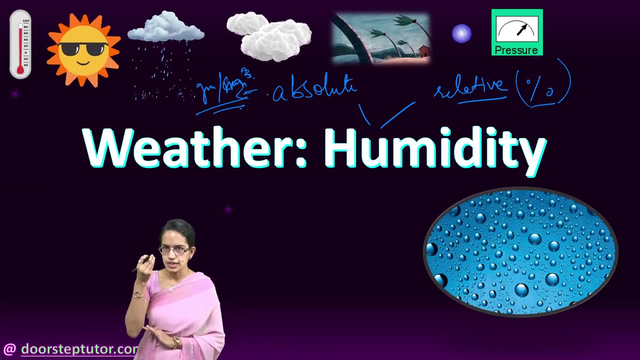 So that is always explained in terms of percentage. very, very important. Absolute is explained in terms of grams per cubic meters. So grams per cubic meters would be absolute. and what is absolute humidity? If I simply want to explain it in words, I can say the actual amount of water vapor present. 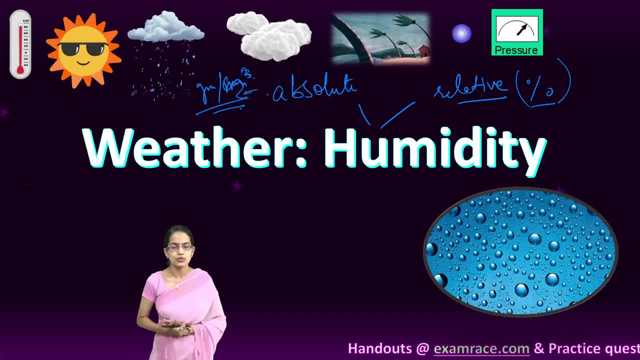 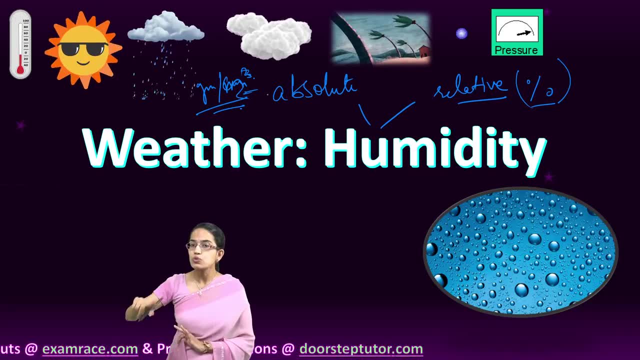 in the atmosphere is what is absolute humidity. relative humidity is the ratio of actual amount of water vapor in the atmosphere. So this is absolute humidity. So total humidity is the ratio of water vapor present in the atmosphere to the total amount of air that a given parcel can hold in a given temperature. 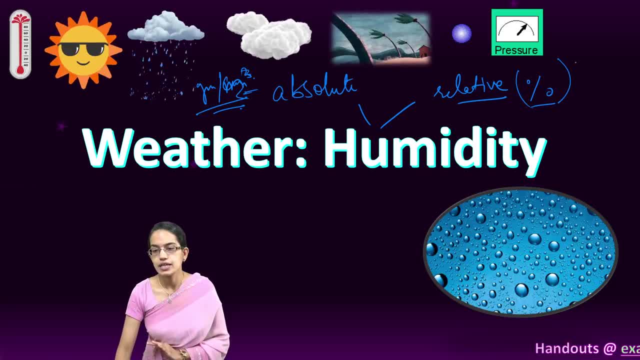 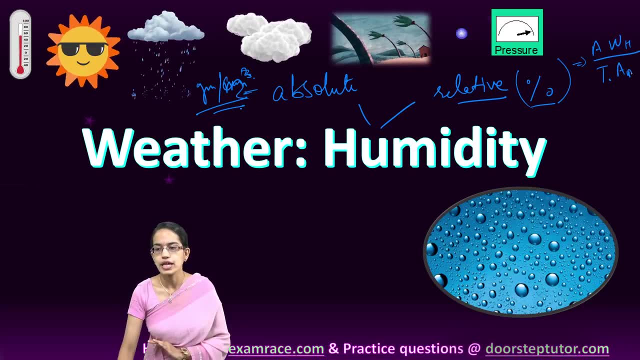 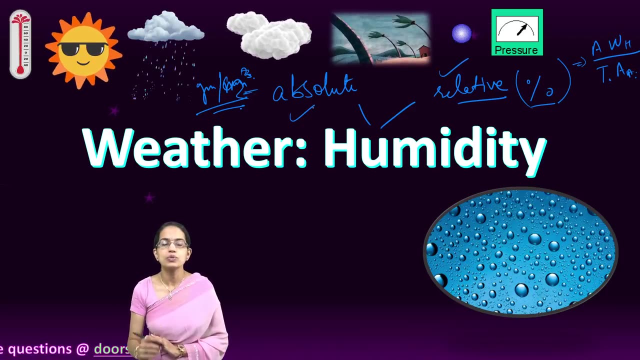 So relative humidity is actual amount of water vapor divided by the total amount of air that is present in a given parcel at a given temperature. so that is relative. Absolute is simply the actual amount of water vapor which is present to the atmosphere, which which is present in the atmosphere and absolute is measured in grams per cubic meters. however, 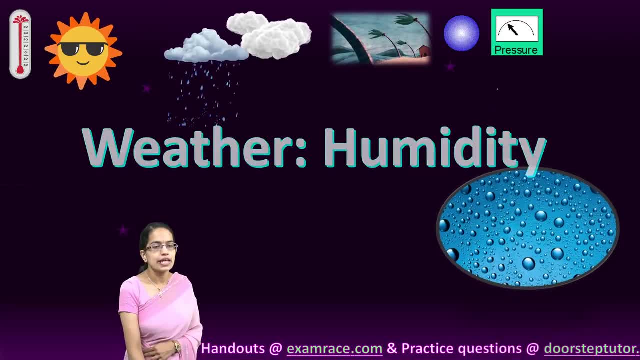 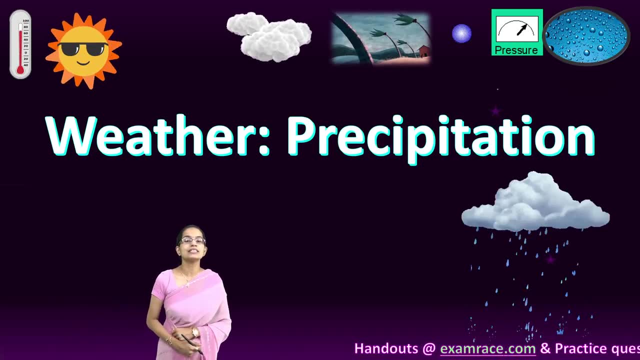 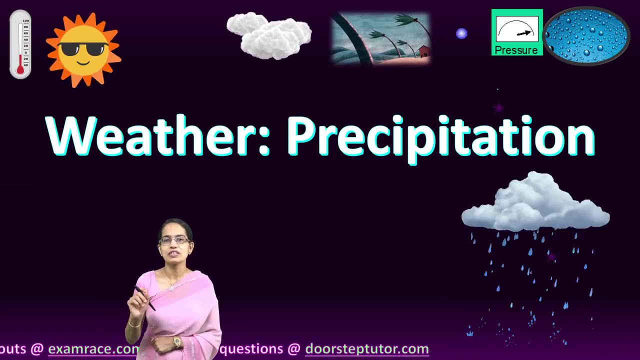 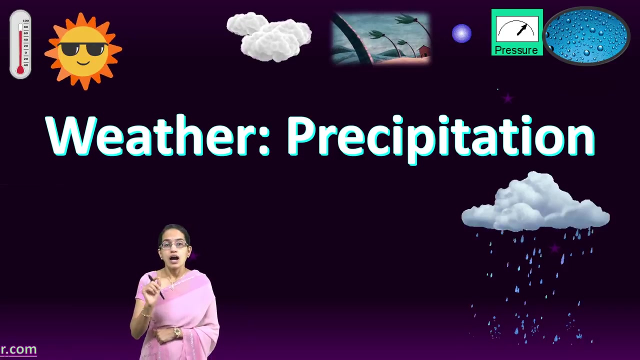 relative humidity is measured in percentage- the next we talk- and humidity is measured through dry and wet bulb thermometer, which we would understand next. the next is precipitation. precipitation or rainfall. now, rainfall is the most common form of precipitation, therefore we say it as rainfall. however, it is incorrect usage precipitation- sorry, can be under various 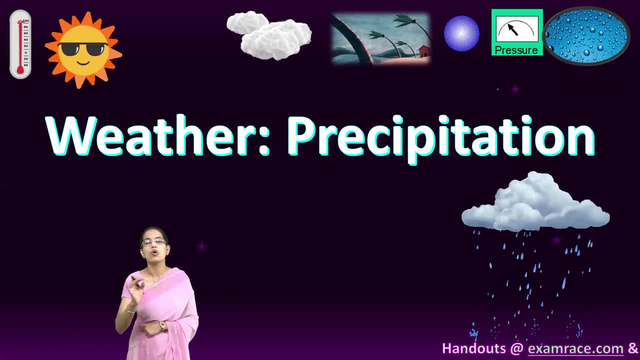 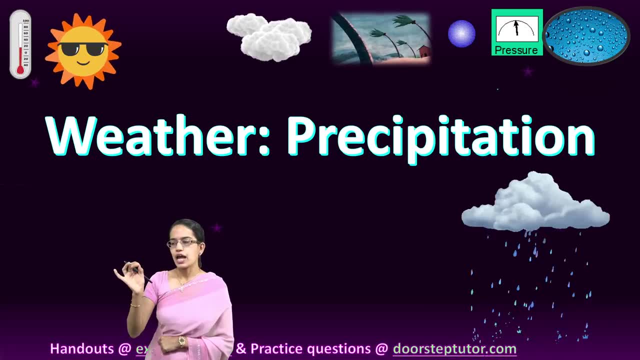 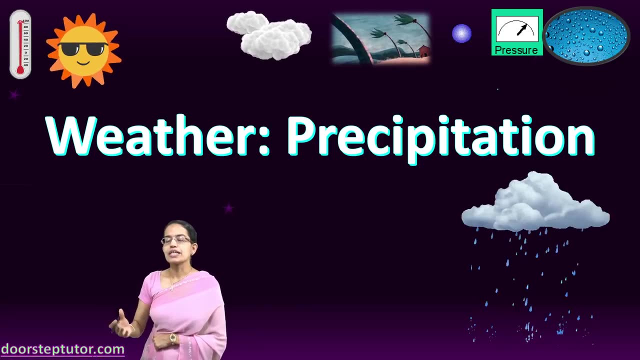 forms, for example, snow, hail, sleet- all of those are forms of precipitation. so precipitation is water, either in solid form or in liquid form, which falls on to the earth surface. now how we explain it? this is simply explained as depositions of at the surface of the earth. 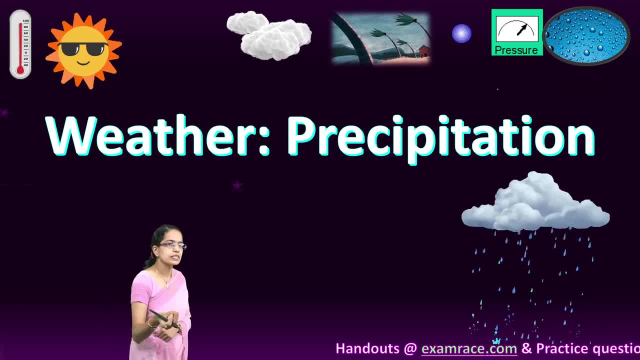 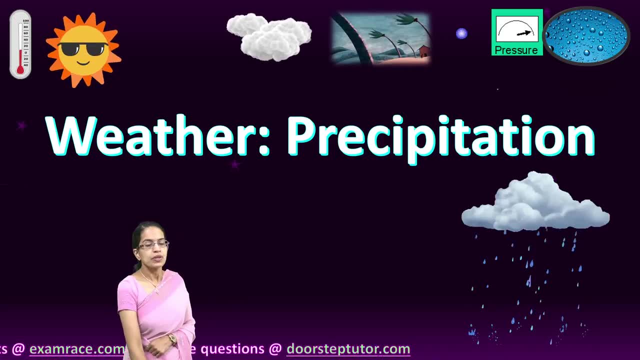 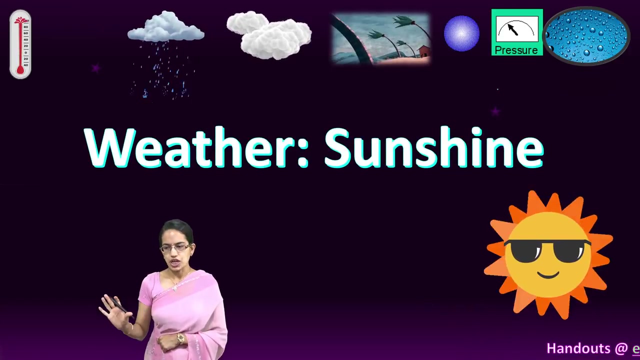 atmospheric moisture and therefore we say this: precipitation is a important part of water cycle or the hydrological cycle. so precipitation is important. rainfall, which is the most common form of precipitation, is measured through rain gauge, which we would understand in the instruments. the next is sunlight: sunshine. now, sunshine is determined by what it is determined. 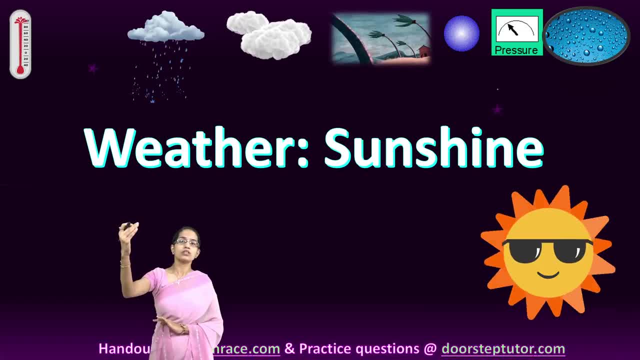 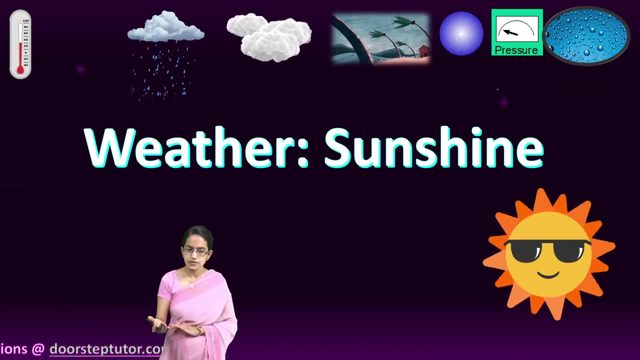 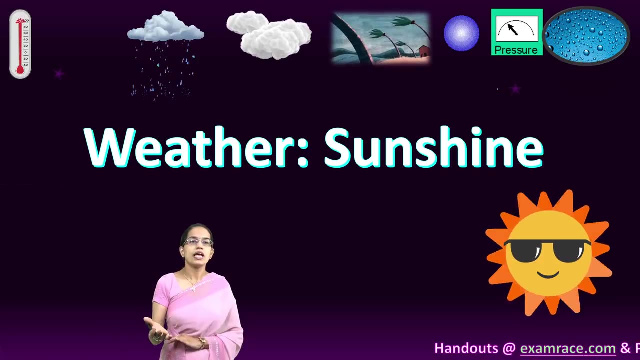 by the latitude you are based on, whether you are on the poles or the equator. places close to the equator or the tropical regions would have higher amount of sunshine. day durations would have higher amount of sunshine in contrast to night and if the phenomena has haze or 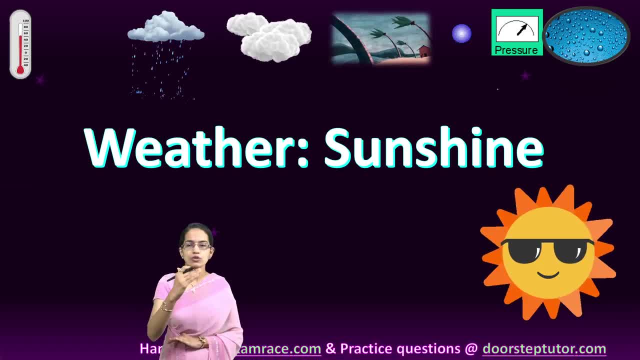 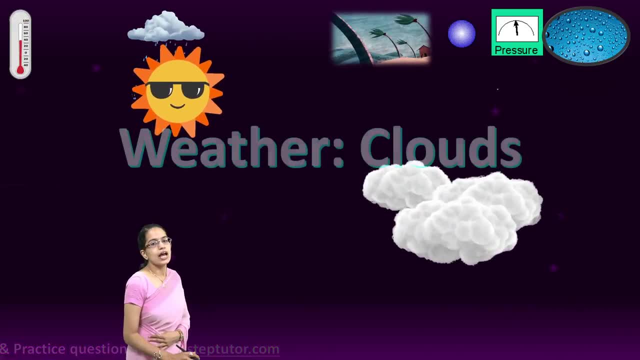 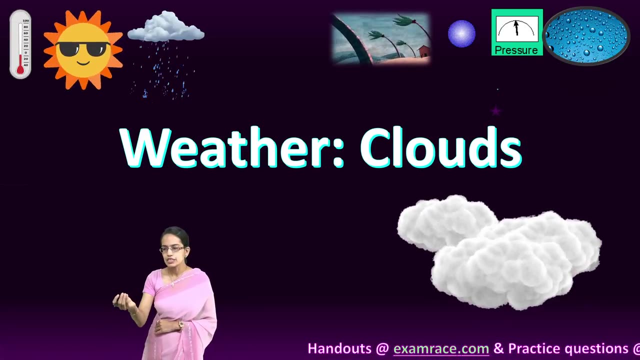 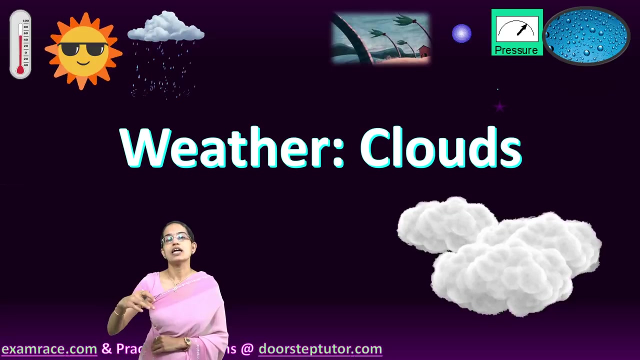 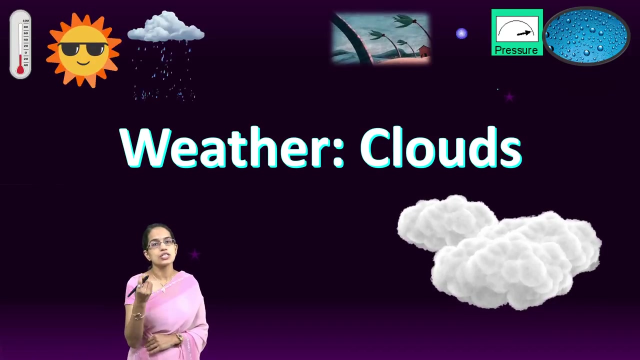 fog or mist, it would definitely reduce the amount of visibility due to reduced sunshine. so sunshine is another important criteria and the last important criteria is the amount of買う, which would make more problematic in холодing environment. now let's show you the temperature of climate environment. 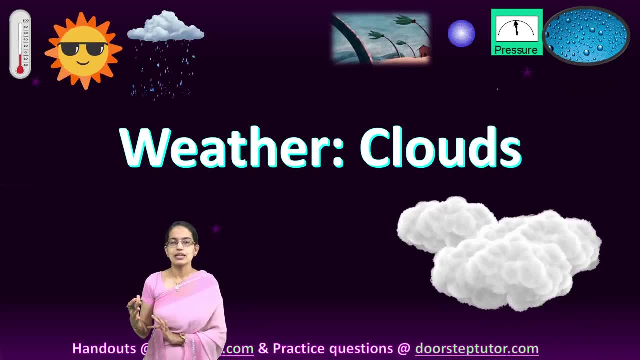 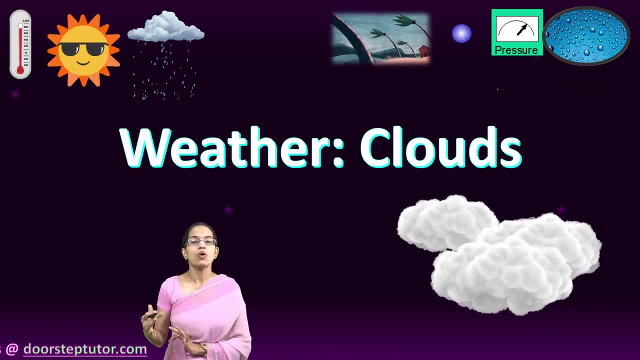 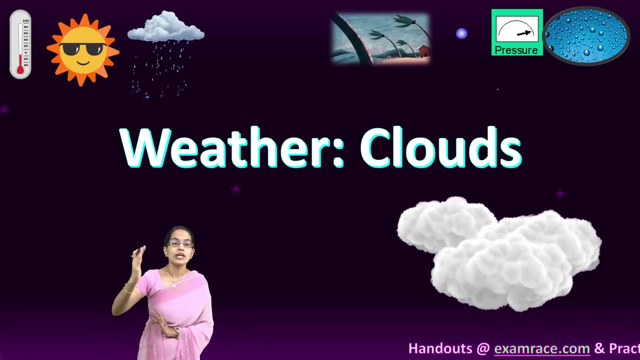 let's see the temperature of climate environment. they can be further dark if they are moisture laden and would have a higher tendency for rain, and these are called as nimbus clouds. we would understand the types of cloud in a while, but sometimes if the cloud is blocking the sunlight, in that case the cloud would appear. 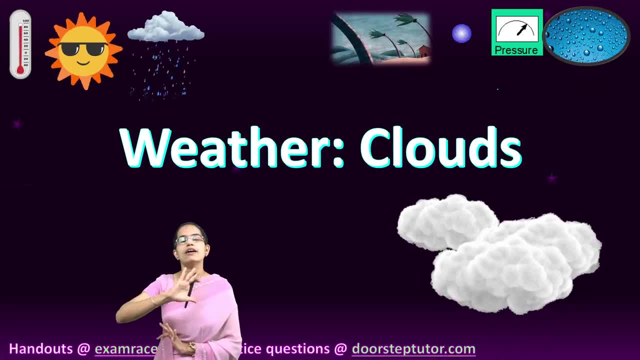 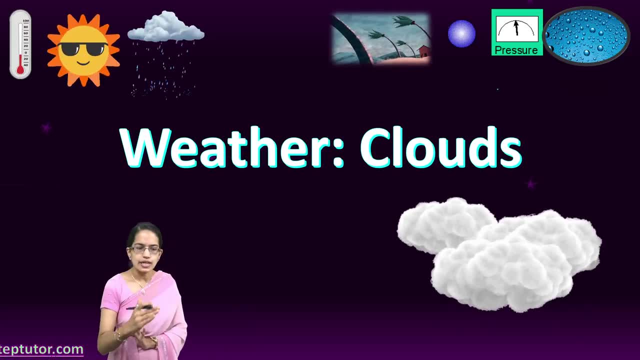 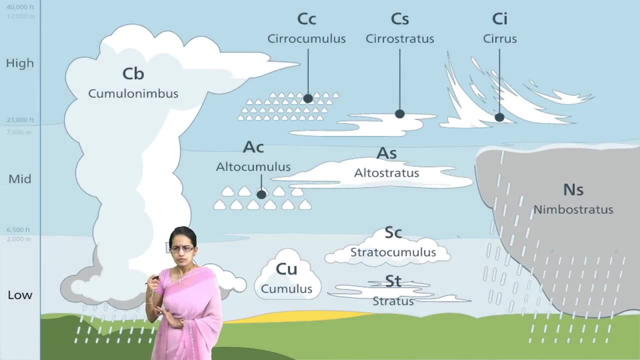 gray. however, if not, the clouds would appear white and they would be able to scatter light much more easily. so that is about understanding the clouds. now, clouds can be classified under various ways, so the first example is a cirrus cloud. cirrus clouds are the highest clouds. they are around 5 to 10 kilometers high, they are feathery in nature and they appear like 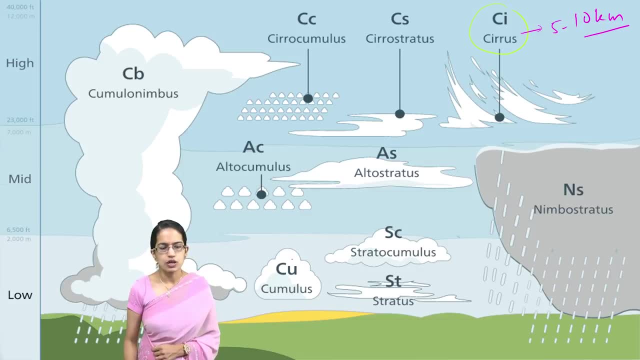 wisp of cotton. the next is cumulus clouds. now, cumulus clouds are similar to cauliflower and they are very high in temperature and they are very high in temperature and they are very high in temperature and they are having a vertical extension as well. but they are also responsible.